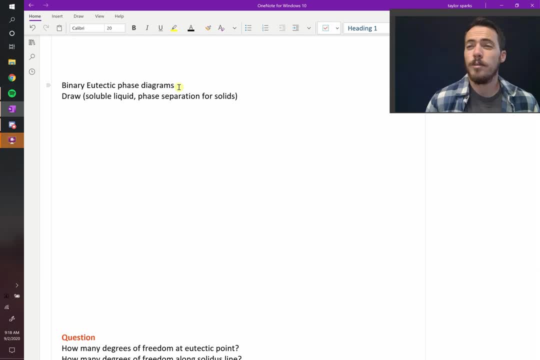 All right, we've talked about an isomorphous binary alloy. That's the simplest binary. Let's go to a slightly more complicated binary. That's the binary eutectic phase diagram. So we call this eutectic because it has a eutectic reaction. A eutectic reaction is: 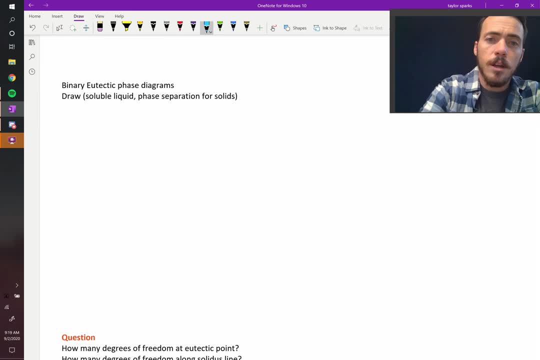 one that has the following reaction: as you cool down, It goes from a liquid and it splits into two different solids, which we'll just call alpha and beta. right, So at a single temperature that reaction takes place, All the liquid disappears and you're left with 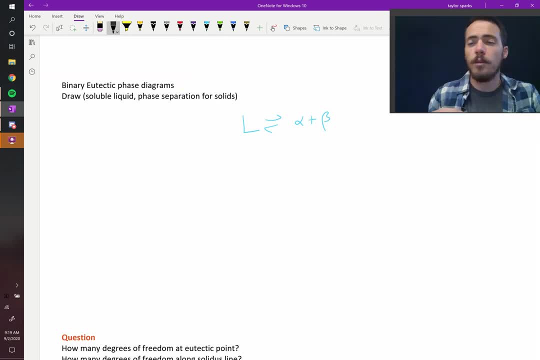 two different solids. So what does our phase diagram look like if it has that reaction? Well, we're going to draw as a function of temperature, All right. so we've got temperature on the y-axis here. On the x-axis, just like before, we're going to have weight percent. 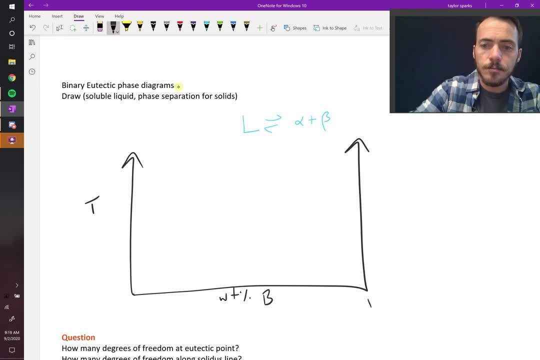 of some component B, right. So we'll put there A and B. And again, A and B can be single elements, but they could also be single elements. So we're going to draw a function of temperature on the y-axis. here And again, A and B can be compounds, right, That could be B could. 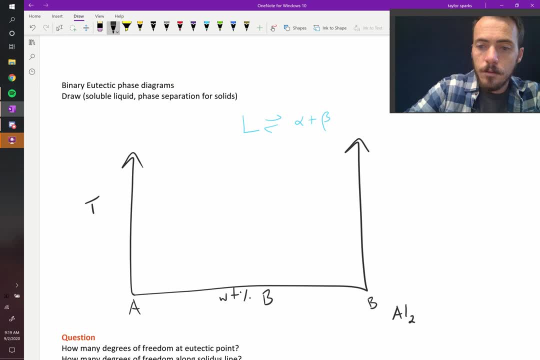 be Al2O3,, for example, And A could be MgO. right, And you could look at as you take MgO and you add Al2O3, you could look at the phase diagram that results or it could be. 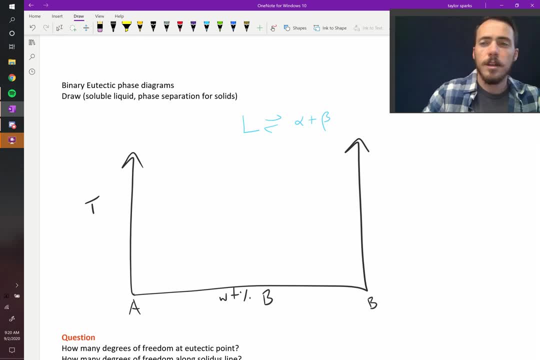 individual elements like lead and tin or bismuth and tin. okay, So if this has a eutectic reaction, it will typically look something like this: Now the exact position of all these points, the lines and the intersections are all. 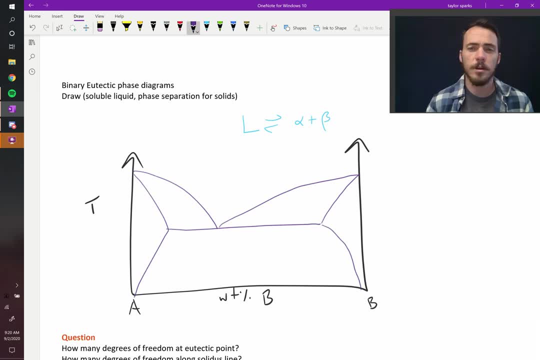 of course, tunable to the exact system that we're considering, but they typically look something like this. Now we need to label these phases. At high temperatures, we're going to have our liquid region up here Now, just like before the isomorphous binary. 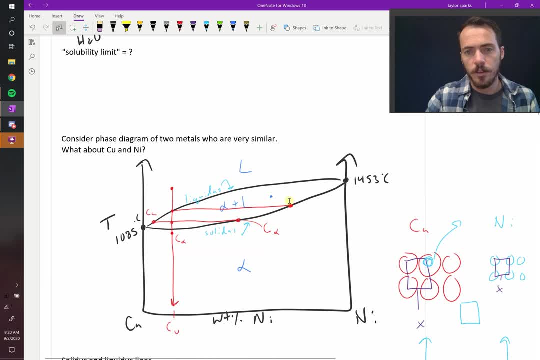 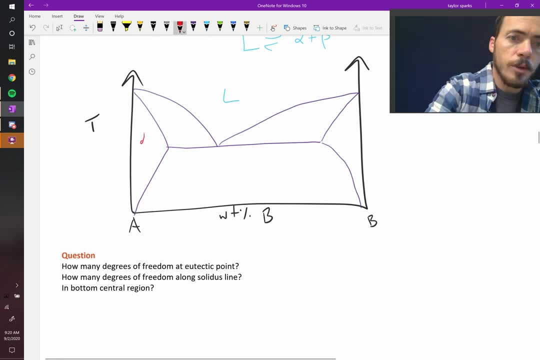 where we had this region of liquid and then we had solid and the region in between them had both. We have the same thing over here. We've got a liquid region and then we have, let's say, a solid region- alpha- over here and a solid region- beta- over here, And that gives us 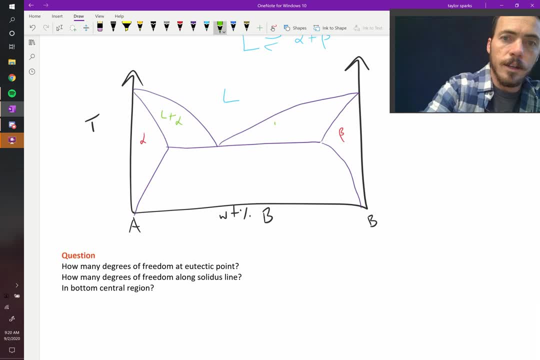 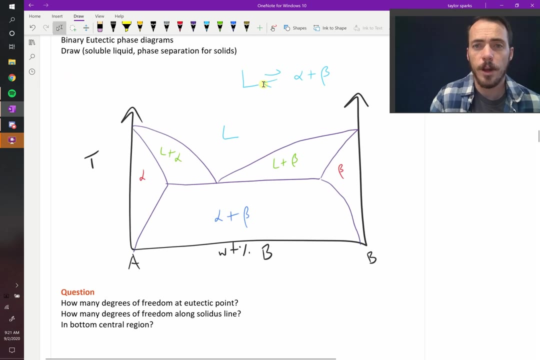 regions like this: liquid plus alpha and liquid plus beta- And then in the middle we have this region where you have alpha plus beta. okay, So can you spot the eutectic, The eutectic point on this diagram where you have this reaction taking place: liquid turning into. 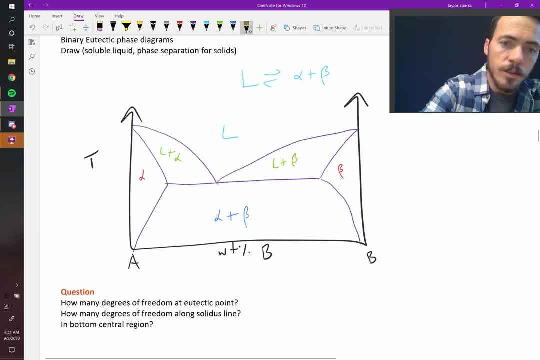 alpha and beta As you cool down. hopefully you can see that it's right here at that point. At that point, as you cool down through that point, if you're at exactly that composition and we call that composition CE for eutectic, usually you would go from a liquid at the CE composition. 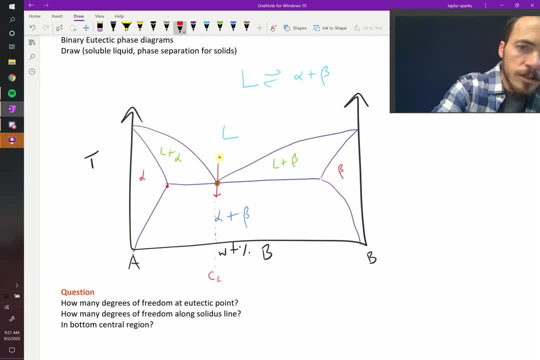 to two solids. Your solid would have this composition over here if it's alpha, and the beta would have that composition over there. So this would be the composition of the alpha phase that forms and this would be the composition of the beta phase that forms. okay, 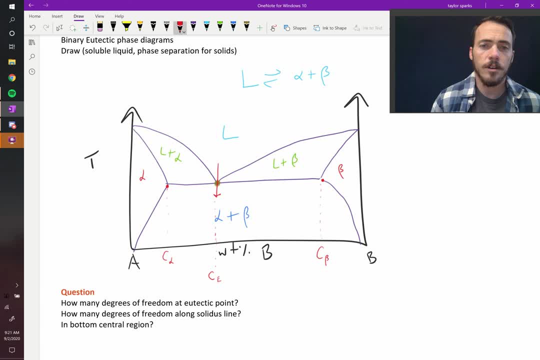 So this is a binary eutectic phase diagram And just like we could do the Gibbs phase rule before, we can apply the Gibbs phase rule here, right? For example, how many degrees of freedom are present at the eutectic point? So at this eutectic point here in the middle, 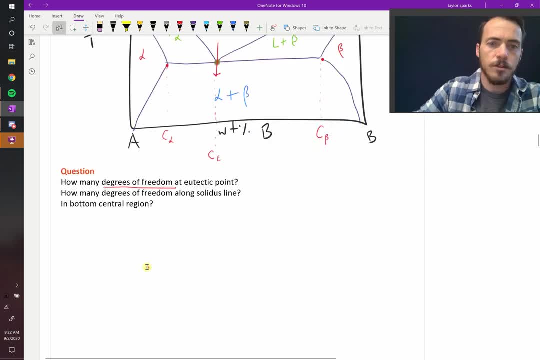 we could apply Gibbs phase rule. So we would say: give ourselves some room. we know that P plus F equals C plus N. So how many phases are present right at that eutectic point? Well, we've got liquid in equilibrium with alpha and beta. 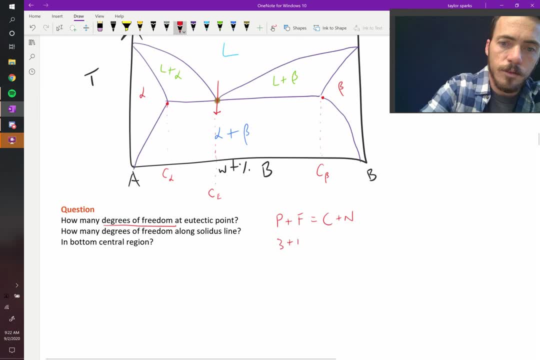 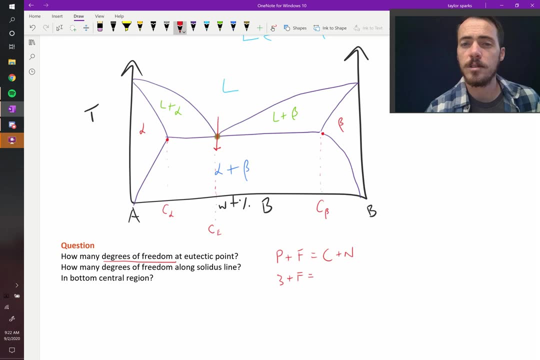 so three different phases. So 3 plus F equals C is the number of components in this system. So how many components do we have? Well, it's going between A and B. so we have two components plus N, where N is the number of non-compositional variables And in this system the only non-compositional 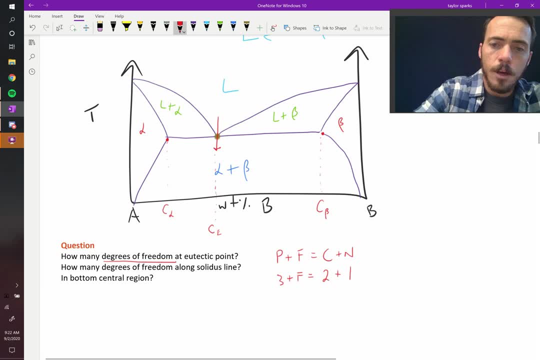 variable is temperature over here, so just one. You could have also made this plot: instead of against temperature, you could make it against pressure. But if you want temperature and pressure, it would have to become a three-dimensional figure which is hard for us to sort of look. 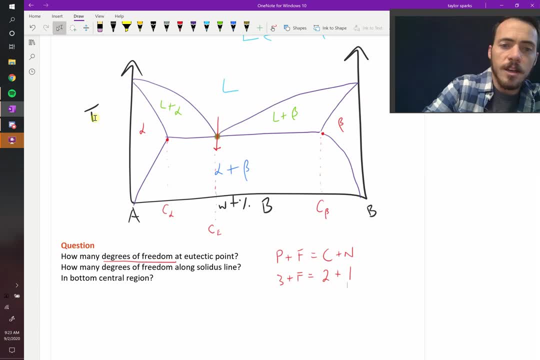 at and interpret, so they usually show these as two-dimensional figures. In any case, you can see that for this case, at the eutectic point F equals zero. In other words, the eutectic point is only one point on the plot, right there where you can have all three.